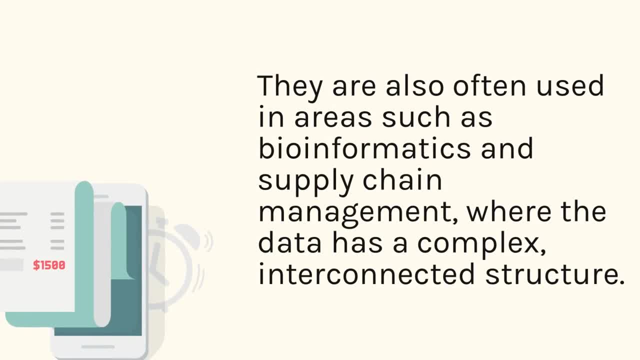 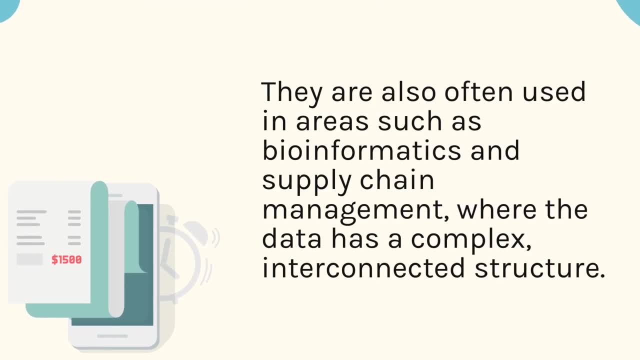 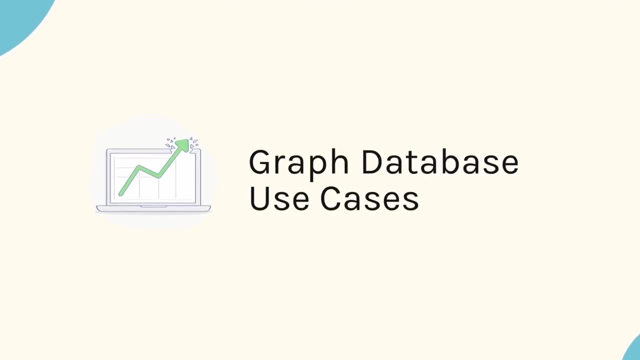 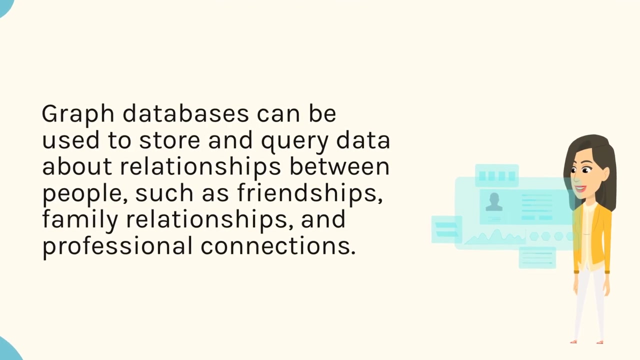 They are also often used in areas such as bioinformatics and supply chain management, where the data has a complex interconnected structure. Graph Database Use Cases. Some common use cases for graph databases include: 1. Social networks: Graph databases can be used to store and query data about relationships between people, such as friendships, family relationships and professional connections. 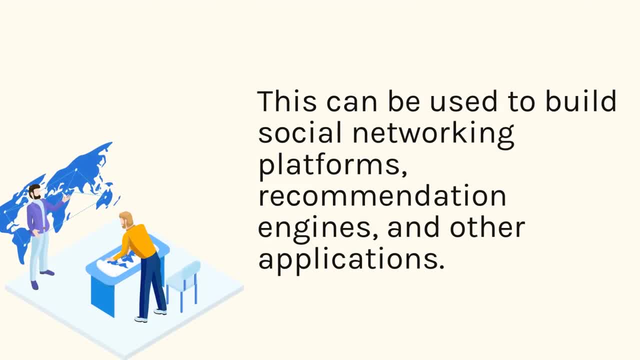 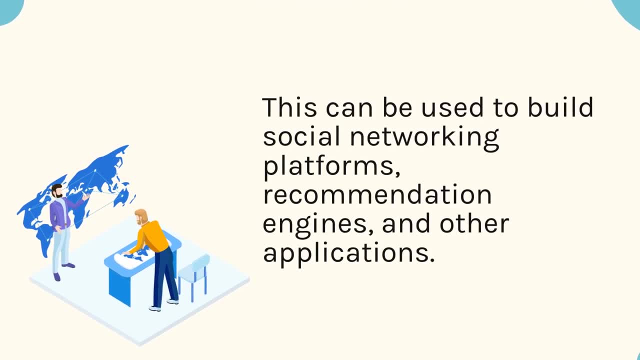 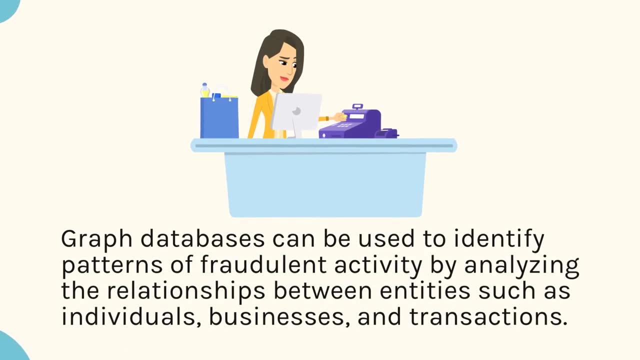 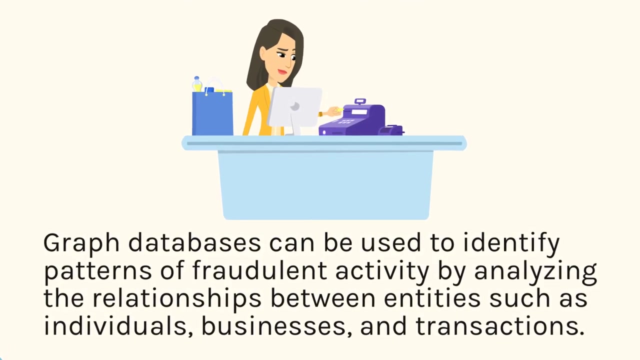 This can be used to build social networking platforms, recommendation engines and other applications. 2. Fraud Detection: Graph databases can be used to identify patterns in a graph database. Graph databases can be used to identify patterns in a graph database. Graph databases can be used to identify patterns of fraudulent activity by analyzing the relationships between entities such as individuals, businesses and transactions. 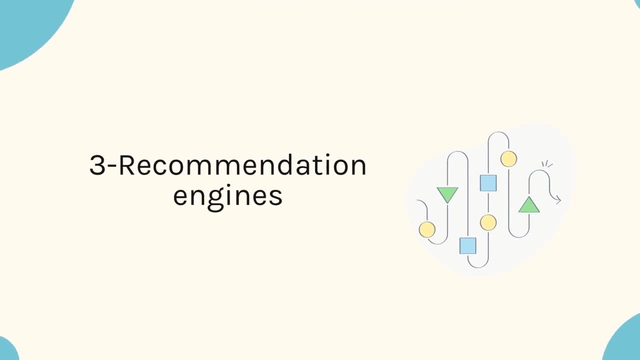 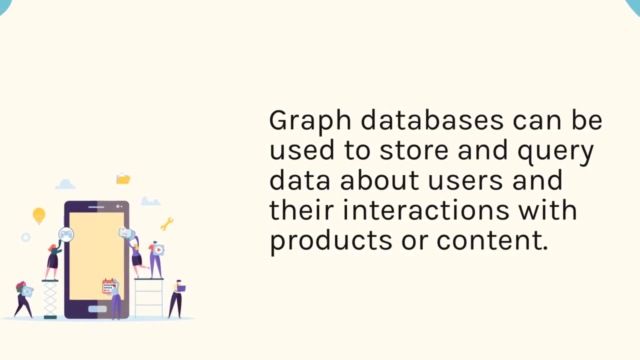 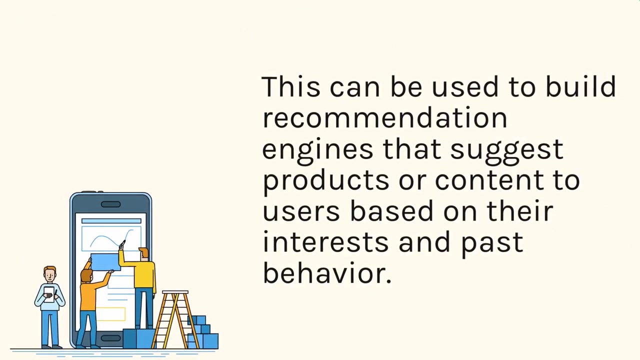 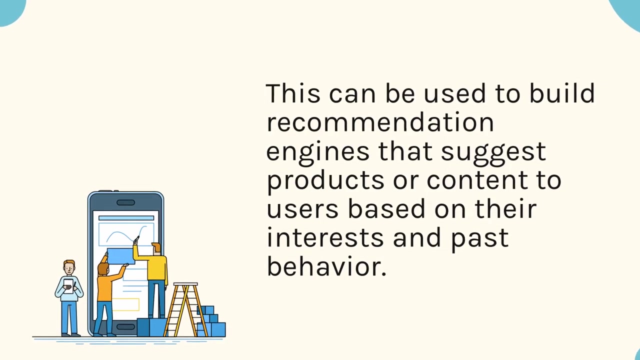 3. Recommendation Engines. Graph databases can be used to store and query data about users and their interactions with products or content. This can be used to build recommendation engines that suggest products or content to users. This can be used to build recommendation engines that suggest products or content to users based on their interests and past behavior. 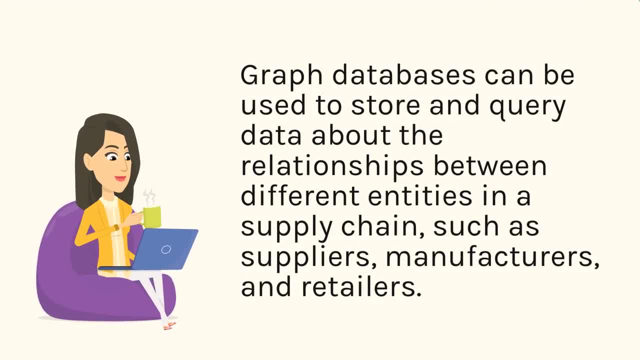 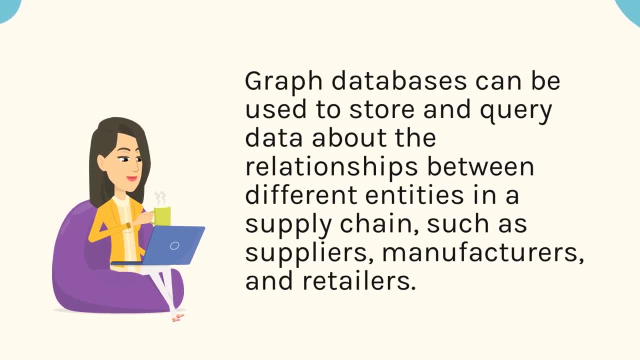 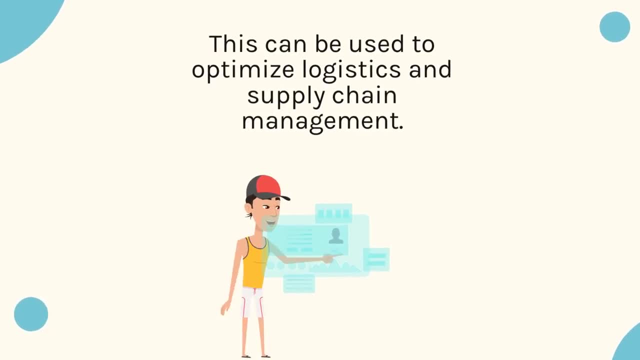 4. Supply Chain Management. Graph databases can be used to store and query data about the relationships between different entities in a supply chain, such as suppliers, manufacturers and retailers. This can be used to optimize logistics and supply chain management. 5. Bioinformatics. 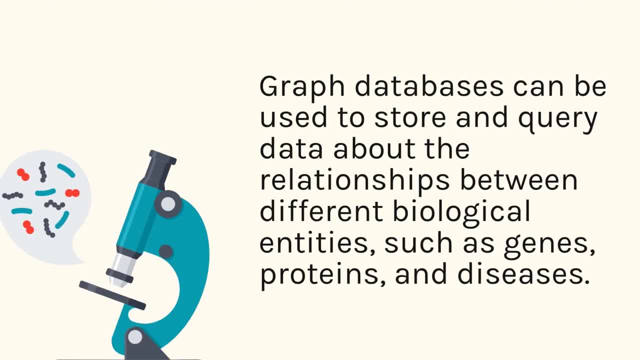 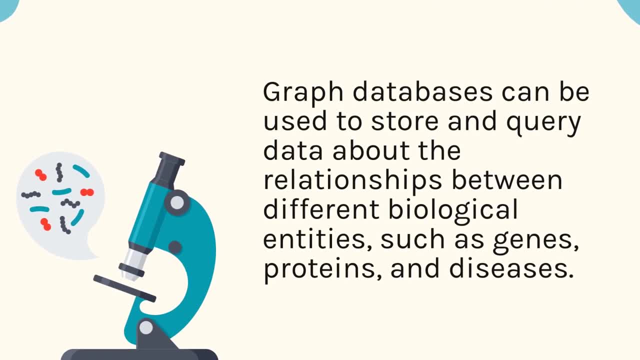 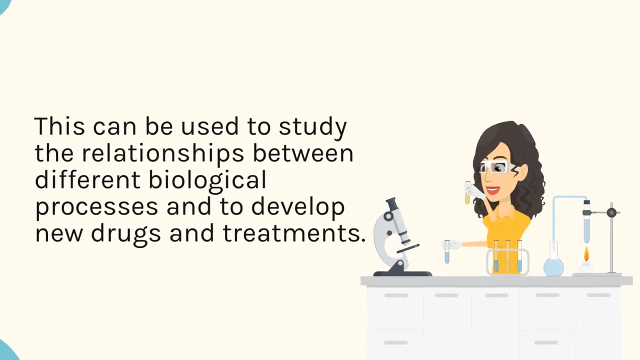 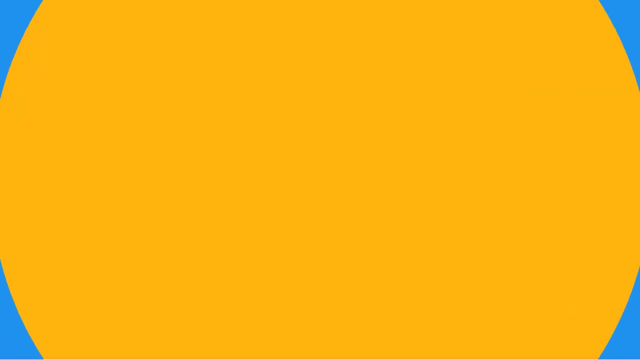 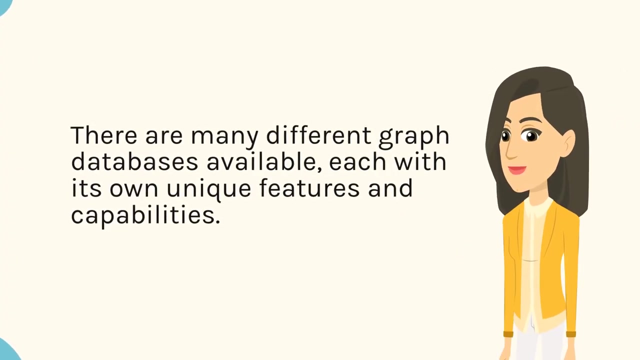 Graph databases can be used to store and query data about the relationships between different biological entities, such as genes, proteins and diseases. This can be used to study the relationships between different biological processes and to develop new drugs and treatments. Graph database list. There are many different graph databases available, each with its own unique features and capabilities. 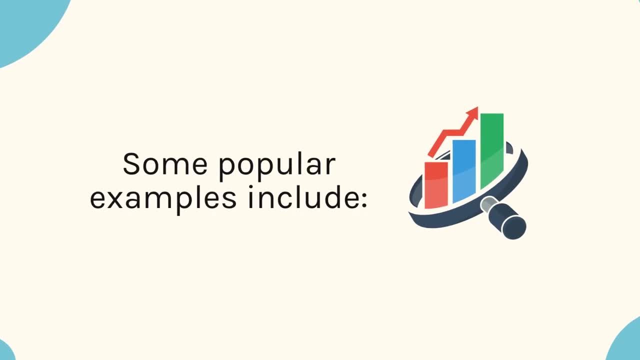 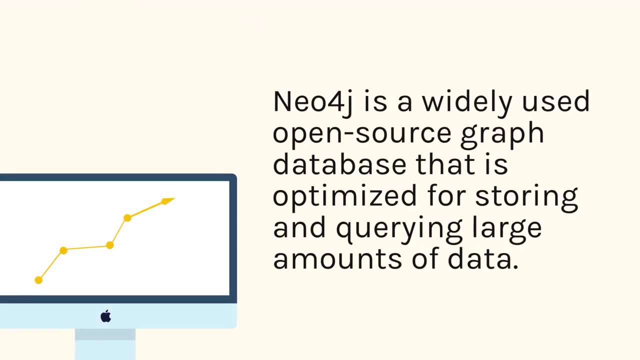 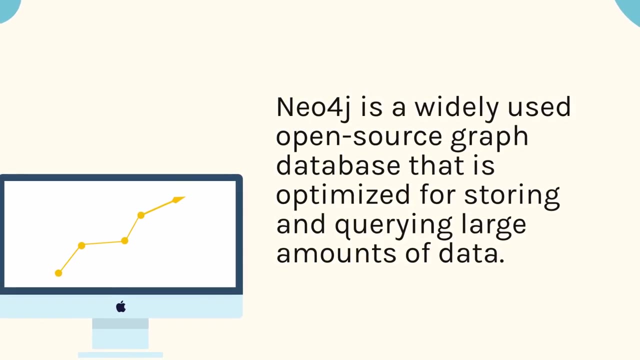 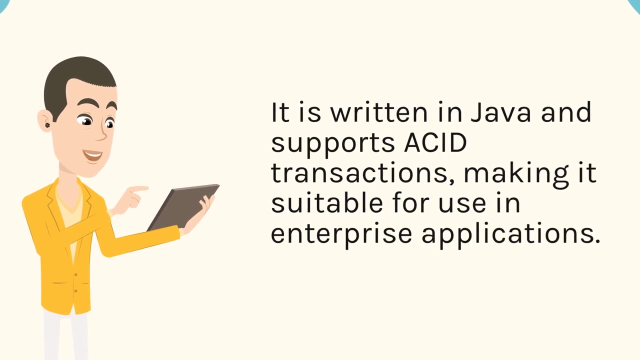 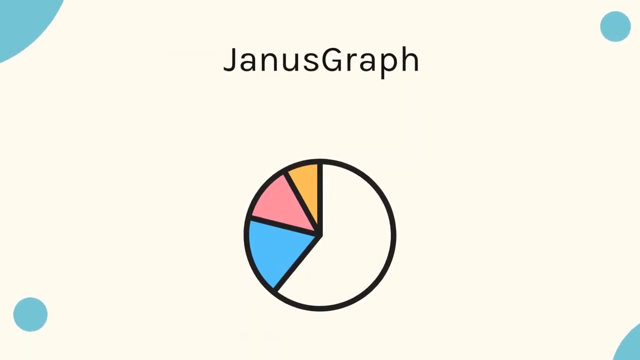 Some popular examples include Neo4j. Neo4j is a widely used open-source graph database that is optimized for storing and querying large amounts of data. It is written in Java and supports ACID transactions, making it suitable for use in enterprise applications. JanusGraph. 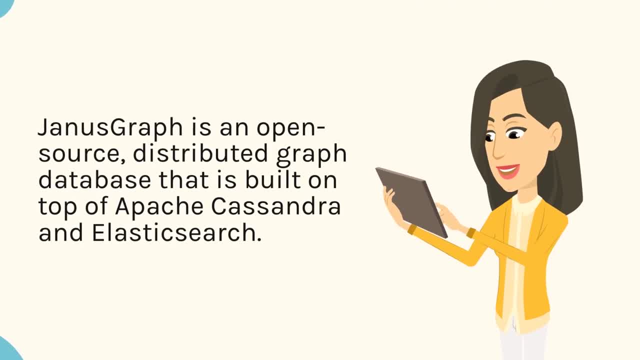 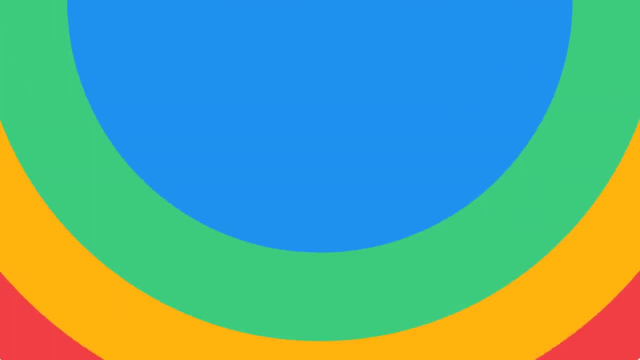 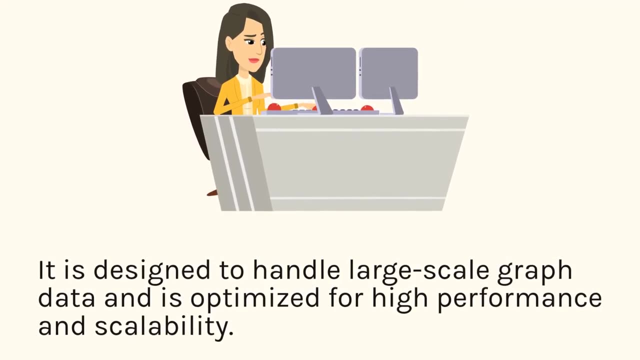 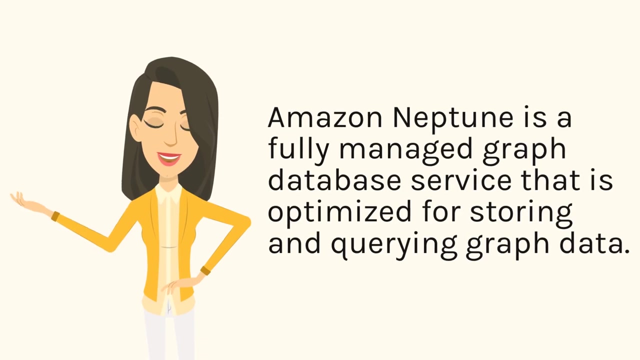 JanusGraph is an open-source, distributed graph database that is built on top of Apache, Cassandra and Elasticsearch. It is designed to handle large-scale graph data. It is optimized for high performance and scalability. Amazon Neptune- Amazon Neptune is a fully managed graph database service that is optimized for storing and querying graph data. 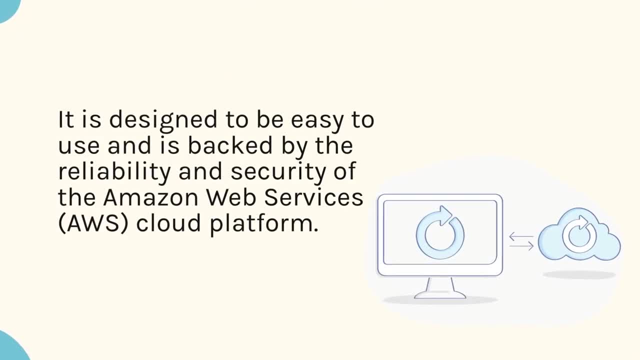 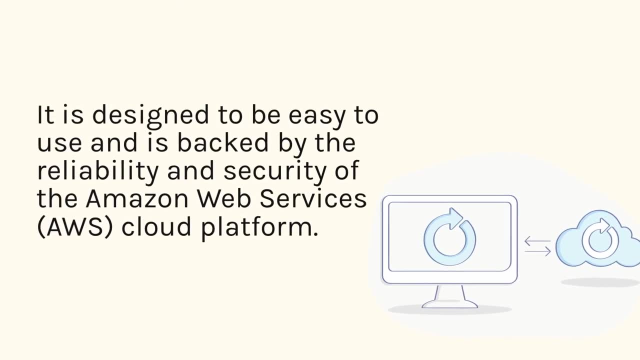 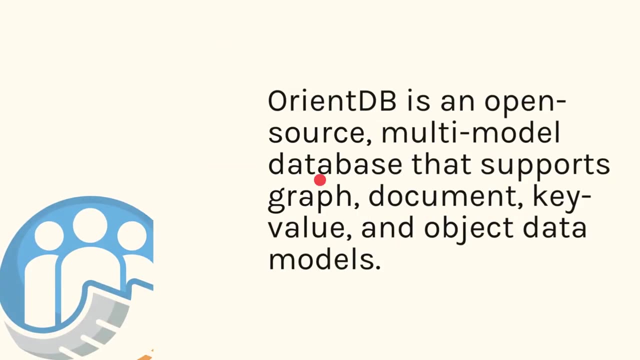 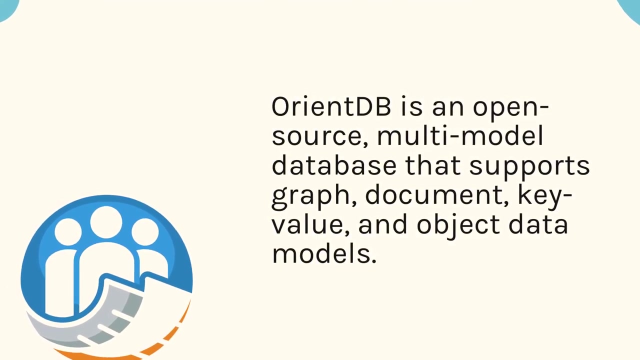 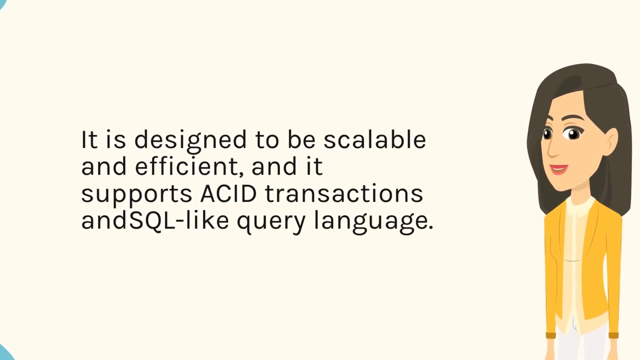 It is designed to be easy to use and is backed by the reliability and security of the Amazon Web Services cloud platform, Orientp. Orientp is an open-source multi-model database that supports graph, document, key value and object data models. It is designed to be scalable and efficient, and it supports ACID transactions and SQL-like query language. 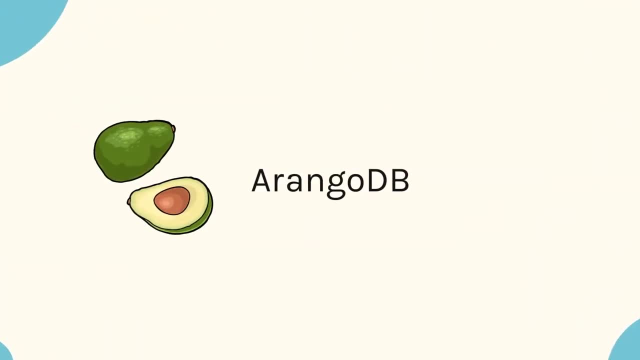 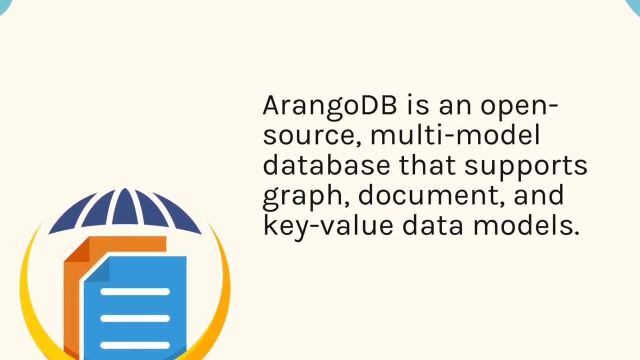 Arangodp. Arangodp is an open-source distributed graph database that is built on top of Apache, Cassandra and Elasticsearch. Arangodp is an open-source multi-model database that supports graph document and key value data models. 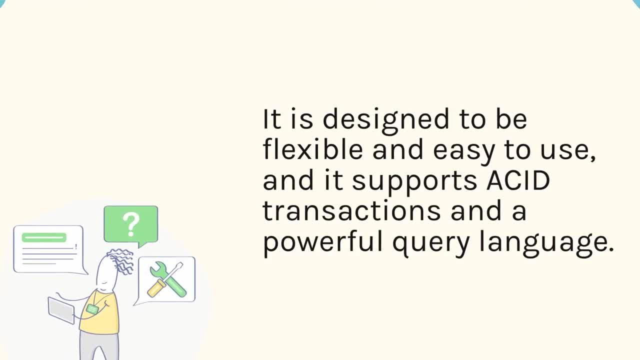 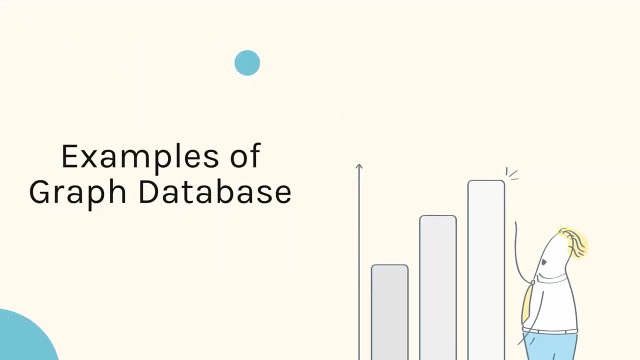 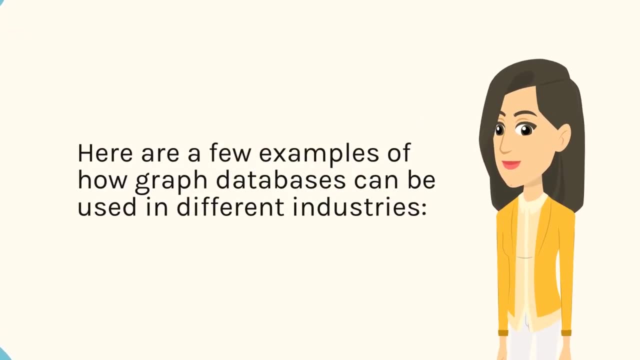 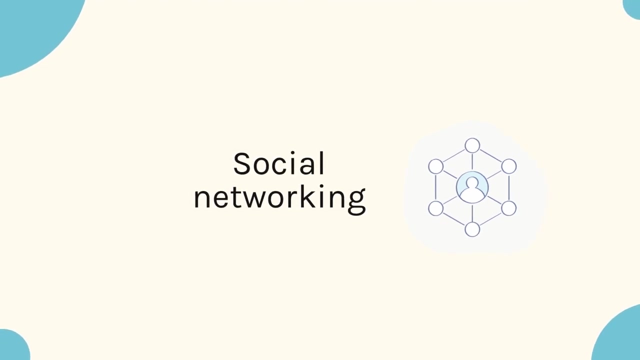 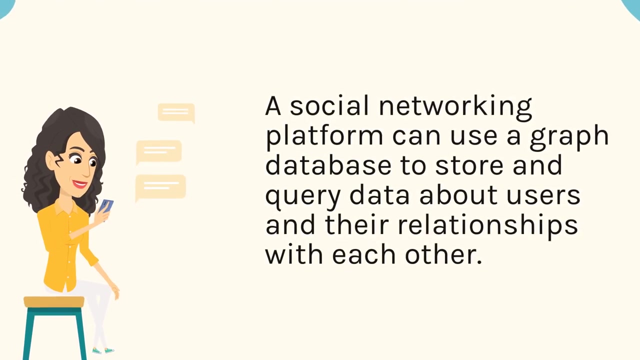 It is designed to be flexible and easy to use, and it supports ACID transactions and a powerful query language. Examples of Graph Database: Here are a few examples of how graph databases can be used in different industries. Social Networking: A social networking platform can use a graph database to store and query data about users and their relationships with each other. 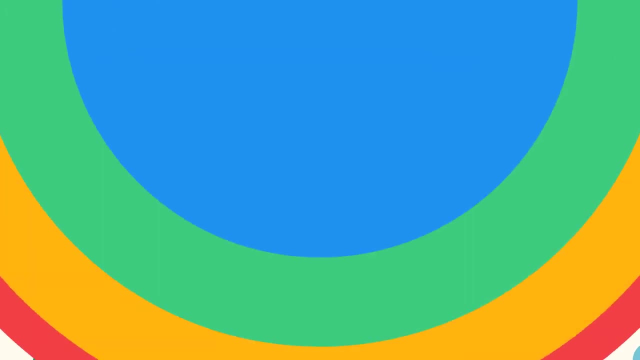 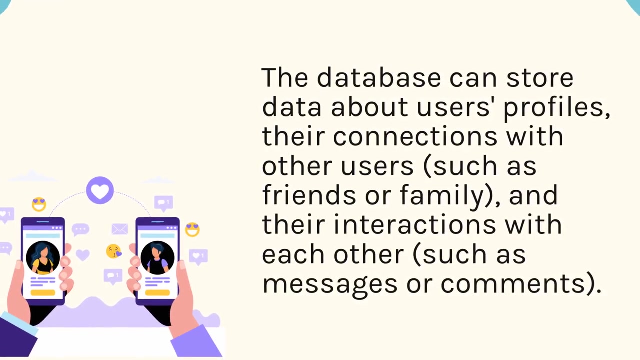 A social networking platform can use a graph database to store and query data about users and their relationships with each other. The database can store data about users' profiles, their connections with other users, such as friends or family, and their interactions with each other, such as messages or comments. 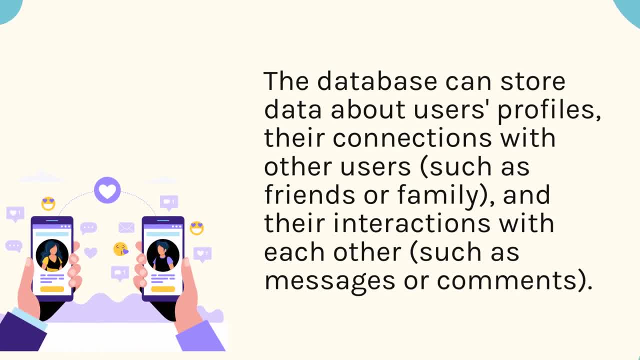 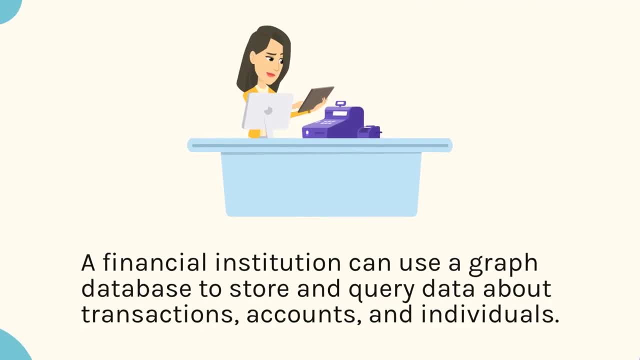 The database can store data about users' profiles, their connections with other users, such as friends or family, and their interactions with each other, such as messages or comments. Fraud Detection: Fraud Detection: A financial institution can use a graph database to store and query data about transactions, accounts and individuals. 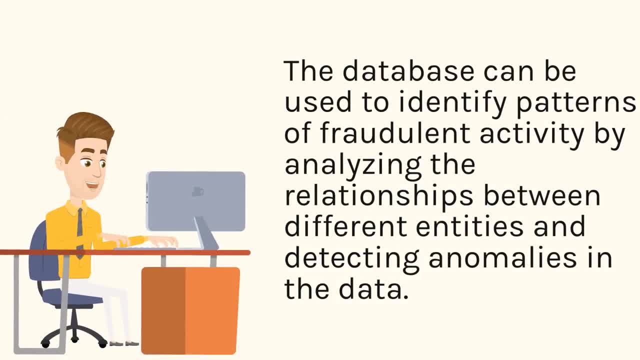 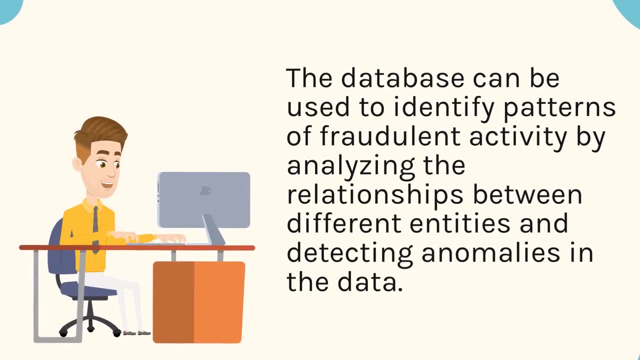 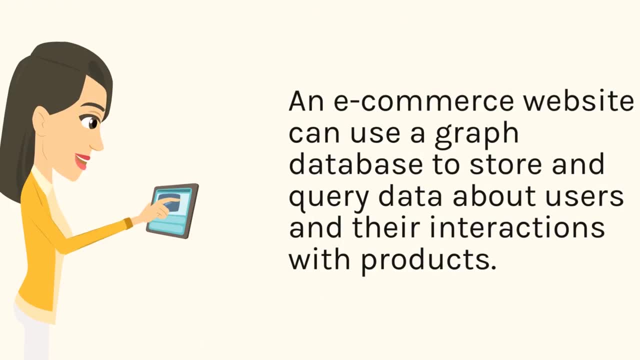 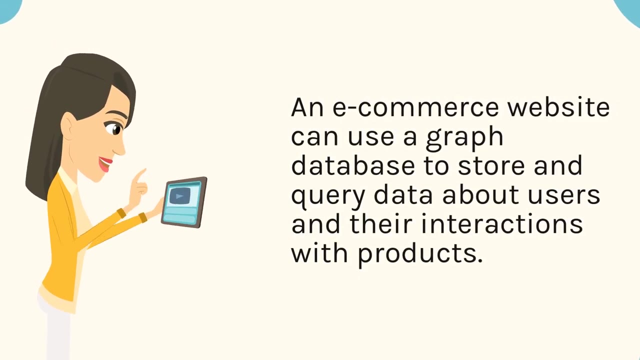 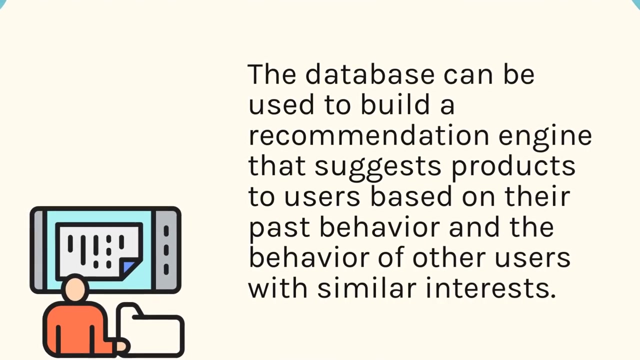 The database can be used to identify patterns of fraudulent activity by analyzing the relationships between different entities and detecting anomalies in the data Recommendation Engines. An e-commerce website can use a graph database to store and query data about users and their interactions with products. The database can be used to build a recommendation engine that suggests products to users based on their past behavior and the behavior of other users with similar interests. 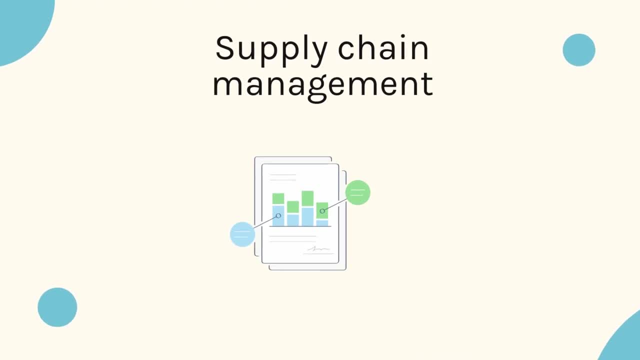 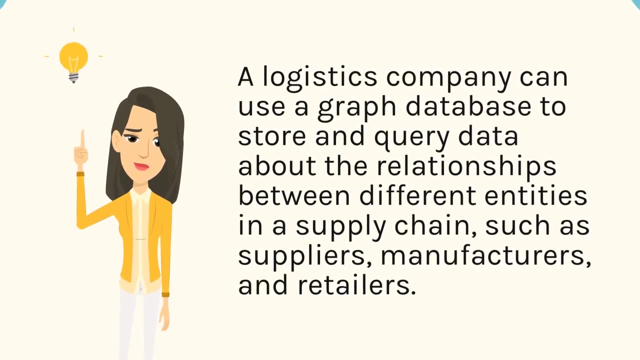 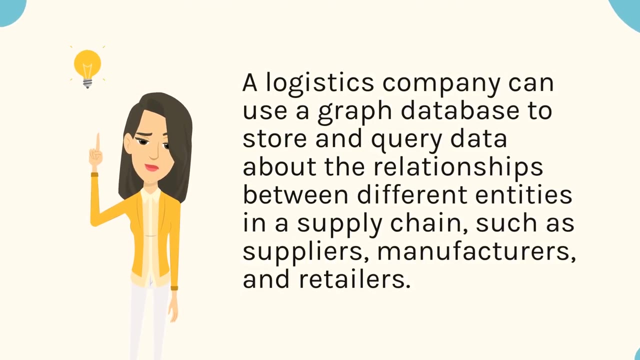 Supply Chain Management. A logistics company can use a graph database to store and query data about the relationships between different entities in a supply chain, such as suppliers, manufacturers and retailers. The database can be used to optimize the flow of goods and improve the efficiency of the supply chain. 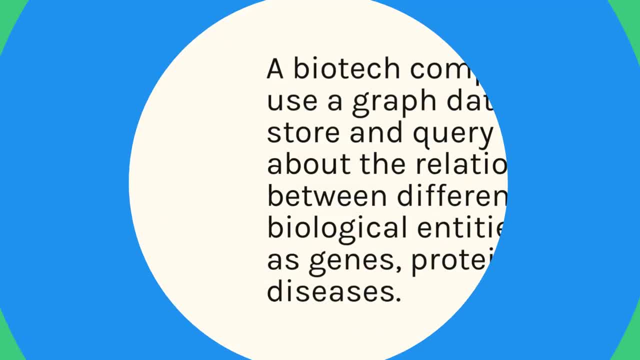 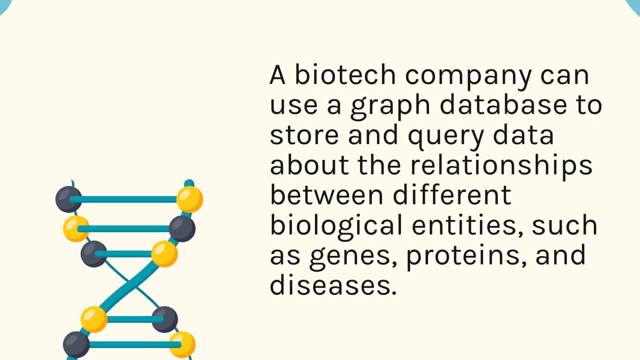 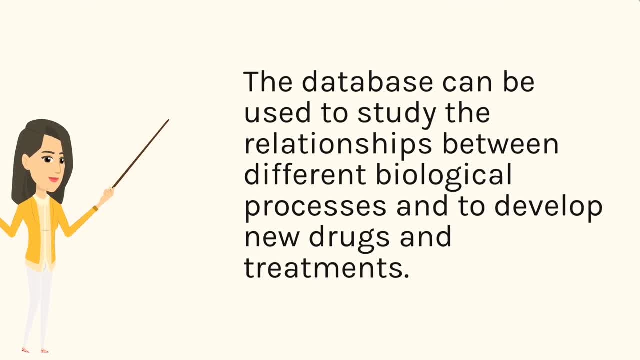 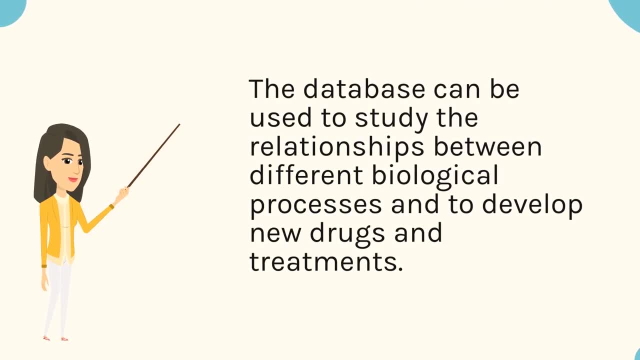 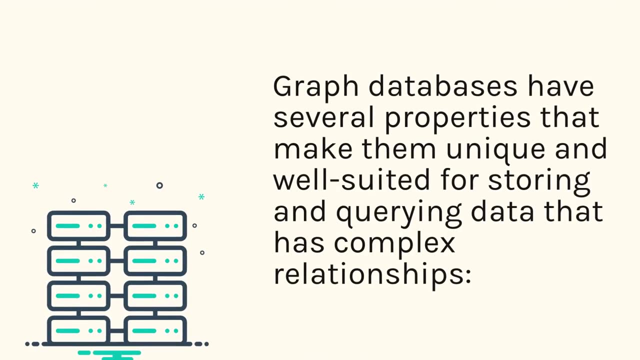 The database can be used to study the relationships between different biological processes and to develop new drugs and treatments. Graph Database Properties. Graph Databases have several properties that may be used to develop new drugs and treatments make them unique and well-suited for storing and querying data that has complex relationships. 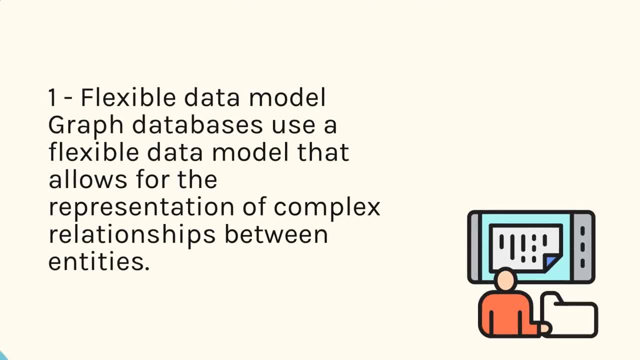 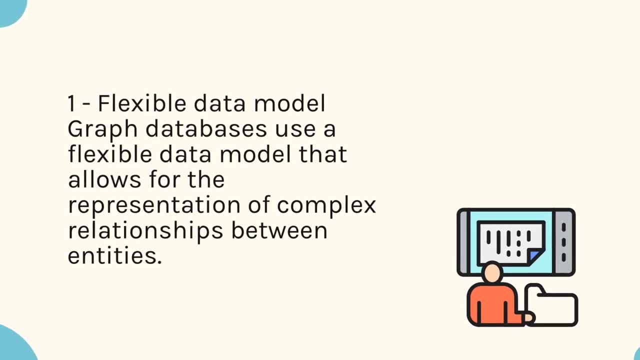 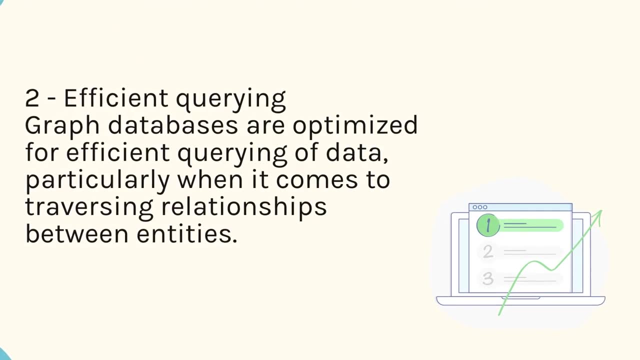 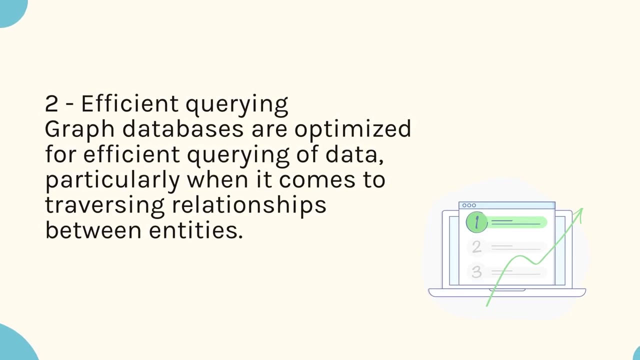 1. Flexible data model. Graph databases use a flexible data model that allows for the representation of complex relationships between entities. 2. Efficient querying: Graph databases are optimized for efficient querying of data, particularly when it comes to traversing relationships between entities. 3. Scalability.